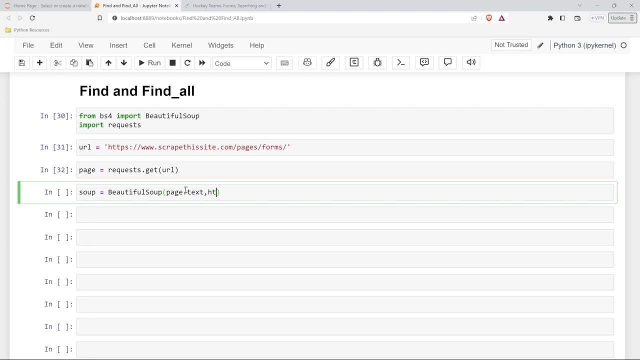 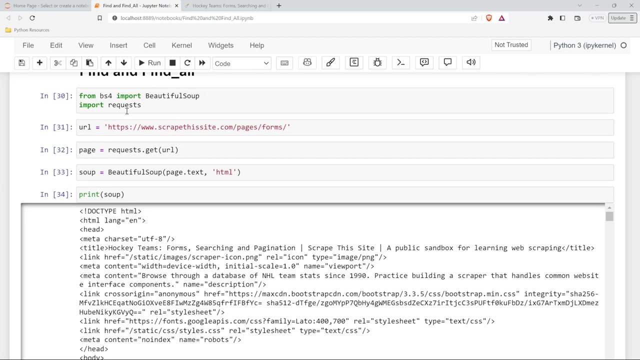 page dot text, because we need that. And our parser, which is HTML, And there we go. And let's go ahead and run this, Let's print it out, make sure it's working, And there we go, So we have our soup right here. All this should look really similar. 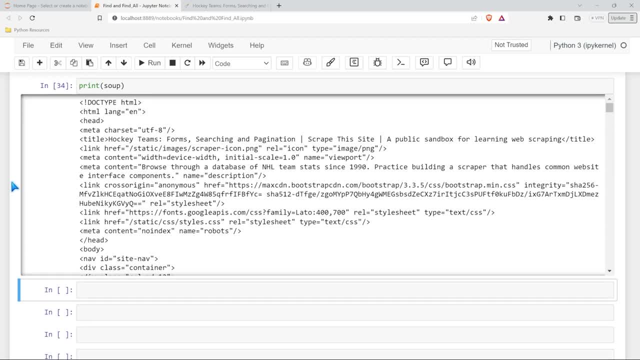 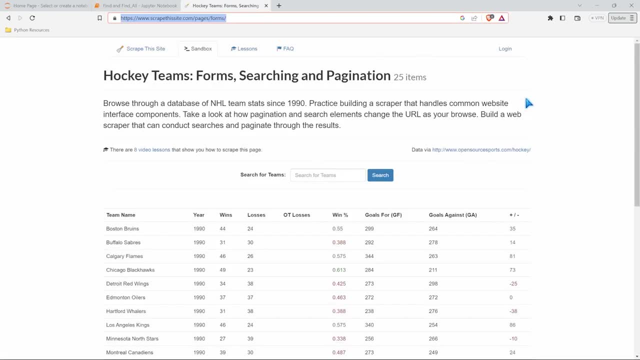 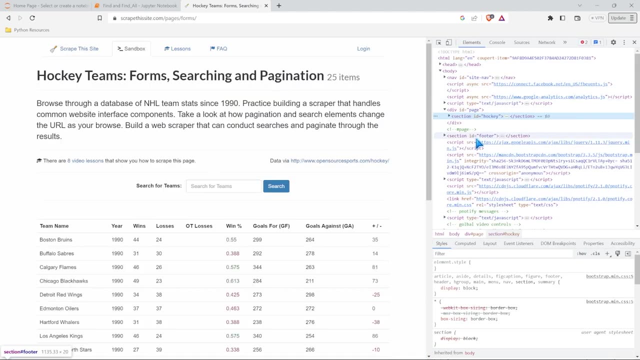 To our last lesson, And so now we've brought in our HTML from our page. We have a lot, a lot, a lot of information here. Now, really quickly, let's come over and let's inspect our webpage Now. in here we have a ton of information, right? We have a bunch of different tags and classes and 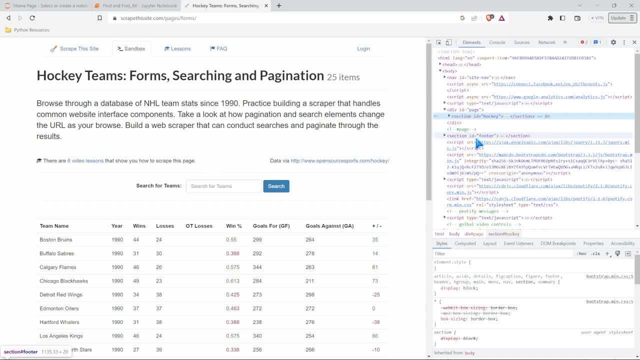 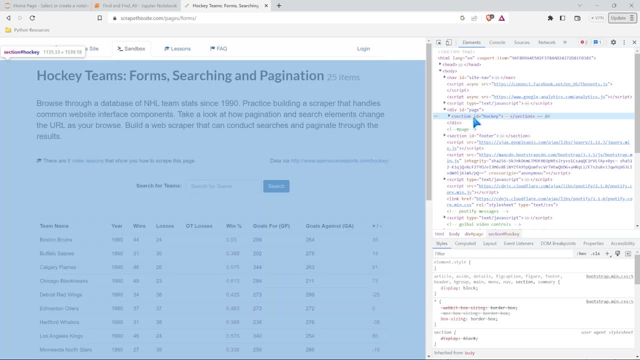 all these other things, but how do we actually use these? Well, that's where the find and find all is going to come into play. And they're pretty similar And you'll see that in just a little bit. But let's say we want to take one of these tags and let's come down. Let's say we just want to. 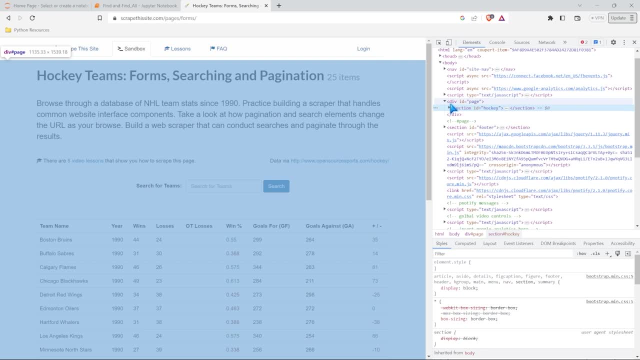 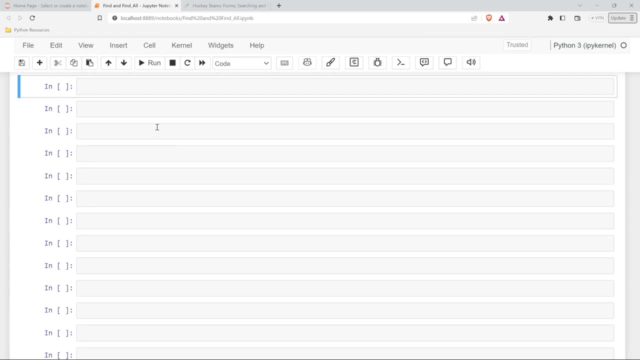 take this div tag. Now, there's gonna be a lot of different div tags in our HTML, But let's just come right here, Let's go down And let's say: we're gonna call soup, we're gonna say soup, that's all. 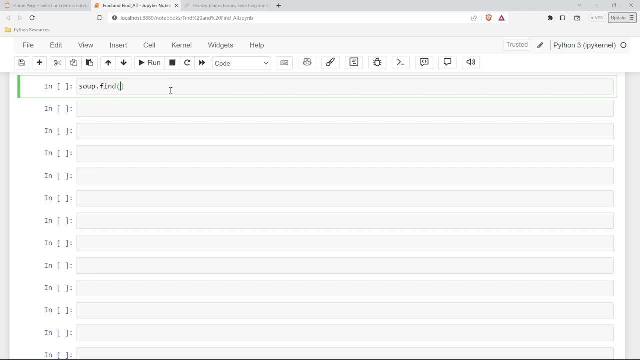 of our information. we're gonna say dot, find. Now, within our parentheses, we can specify a lot of different things, But we're gonna keep it really simple. right now, we're just gonna say D I, V. let's go ahead and run this. What this is going to bring up is the very first div tag in our HTML. 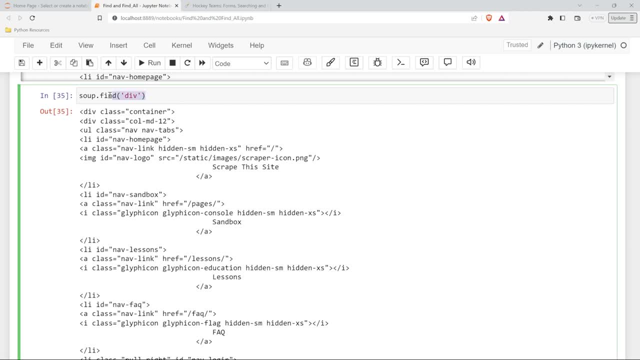 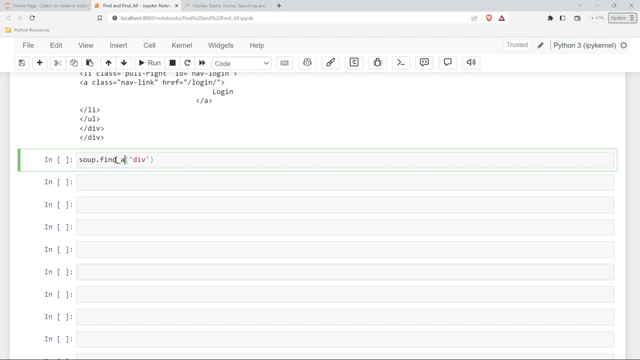 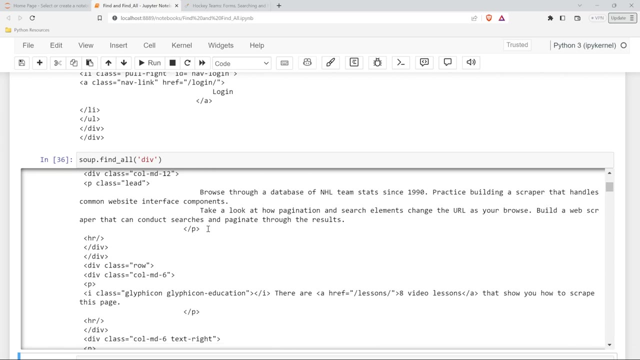 And that's gonna be this information right here. Now let's copy this. I'm going to do the exact same thing, Except we're going to say find underscore, all. Now, let's run this. Now we're going to have a ton more information. Really, all find and find. all do is that they find the. 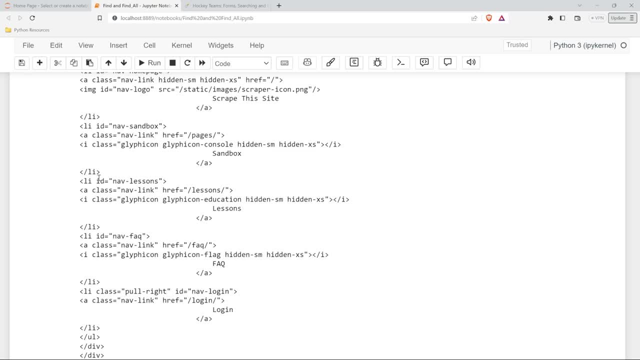 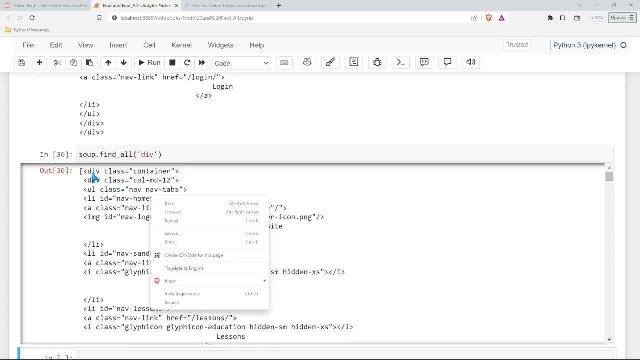 information. now, find is only going to find the first response. Now let's go ahead and run this In our HTML. at least that's the div class container, And let's go back up to the top. That's our div class container. But find all is going to find all of them, So it'll put it in this. 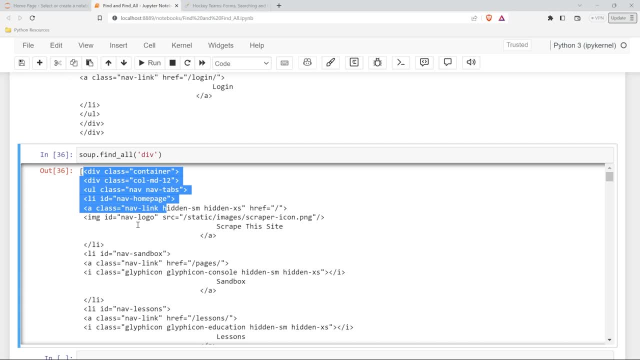 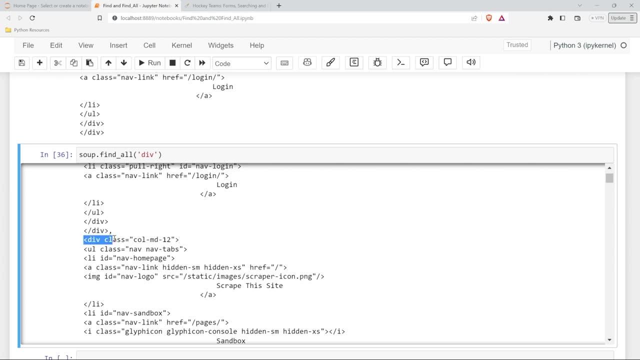 list for you. So it's going to have this first one and it goes down to this forward slash div, which should be right here, And then we have a comma which separates our next div tag. So that is how we can use it. Now, what if we want to specify one of these div tags? we pulled in a ton. of them, But we want to just look for one of them, So let's go ahead and run this Now. let's go ahead and run this And we'll see what happens. So let's just type in this div tag. this is just one of. 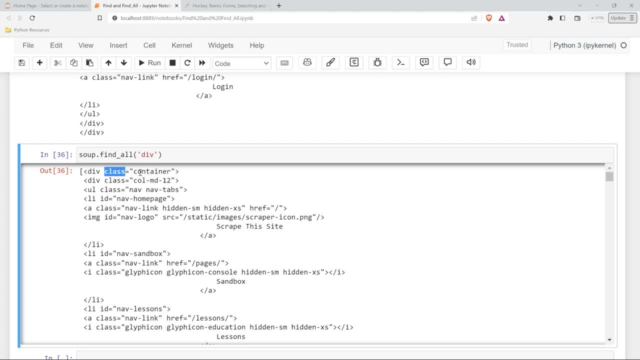 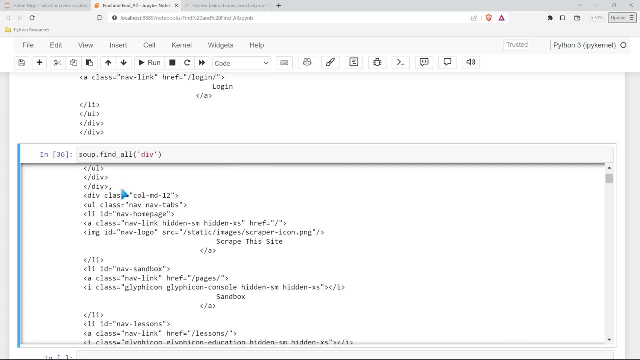 them. Well, this is something where the class comes in handy, because right now we have: class is equal to container, class is equal to col MD dash 12.. I don't know what these are at the off the top of my head, But usually they'll be somewhat unique And we can use these to help us specify. 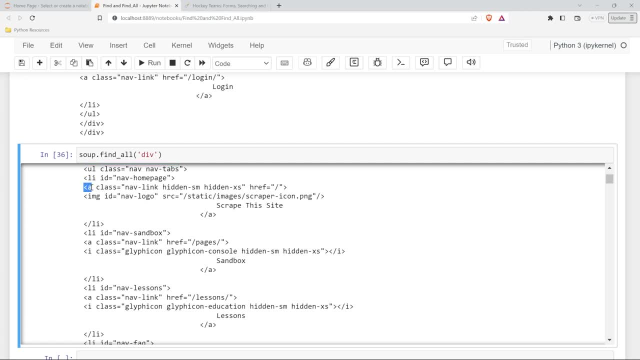 what we're looking for. For example, just kind of glancing at this, we can also use this a tag if we wanted to look at this So we could say, Oh, we're looking for these h refs, So we have an h. 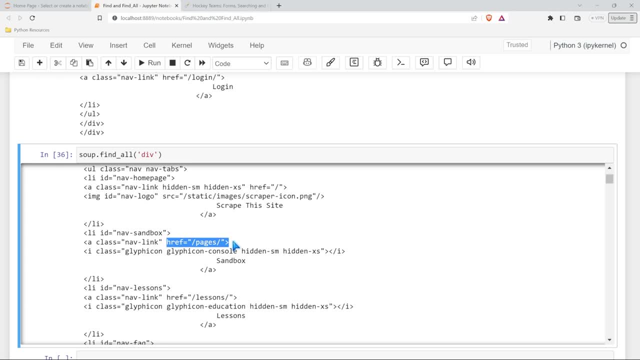 href here And this right down here. we have this href as well, which, again, if you remember from previous lesson, that stands for a hyperlink, Now something like the class or the href or these IDs. these are all attributes So we can specify or kind of filter down based. 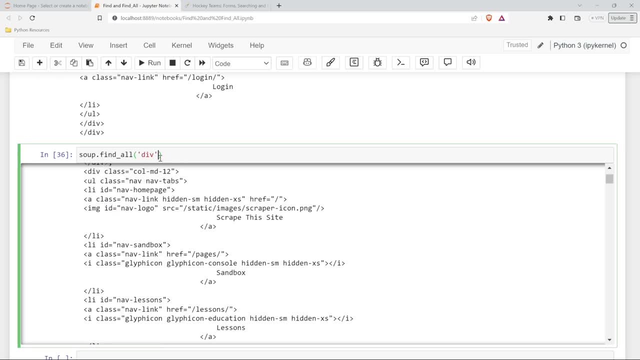 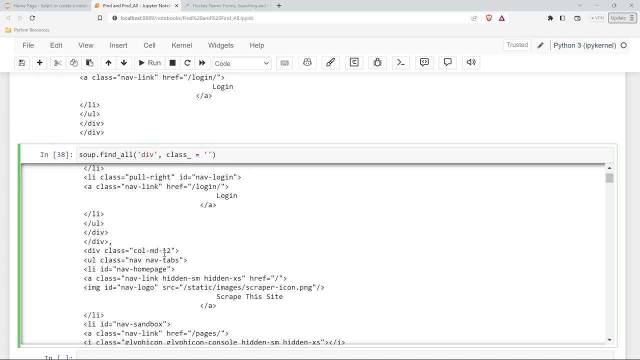 off of these. Now let's try it. So what we can do is we can do class first, And this is kind of the default within something like find all is you can even do class underscore. we can come right back up, we have this div and then here's our class. So again we have 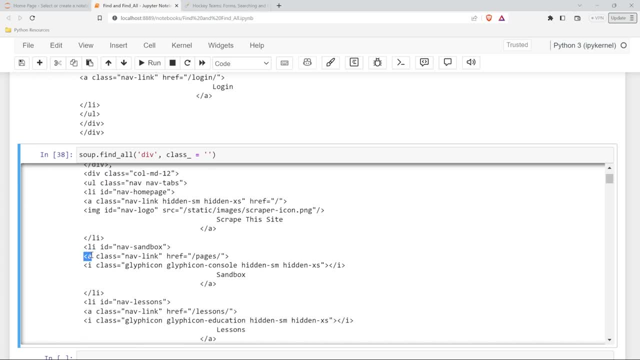 to have the div and the class. if we took this a tag, this is an a tag which would go right here with the class of something like nav link or something like nav link Again down here we need to specify that more. But we have our div, So we'll say class: call MD 12,. 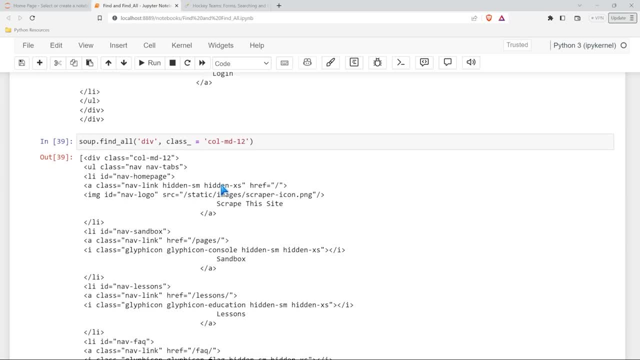 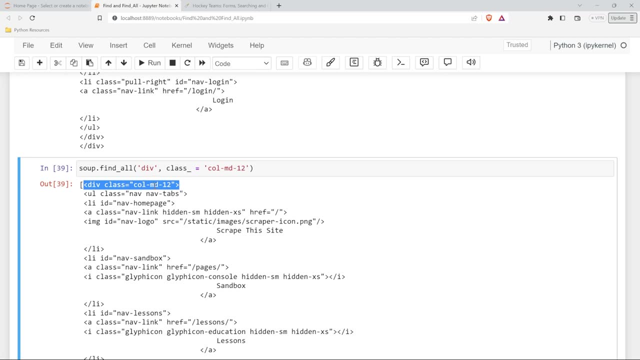 right here And let's go ahead and run this. And now it's going to pull in just that information. Now we're still getting a list because we have multiple of these. So this div we're going to give class call MD dash 12 doesn't just happen once. if we scroll down, we'll. 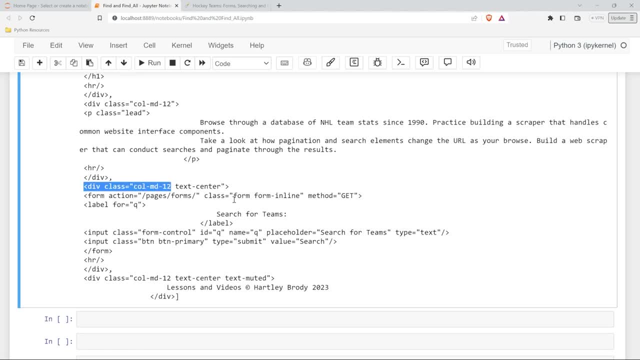 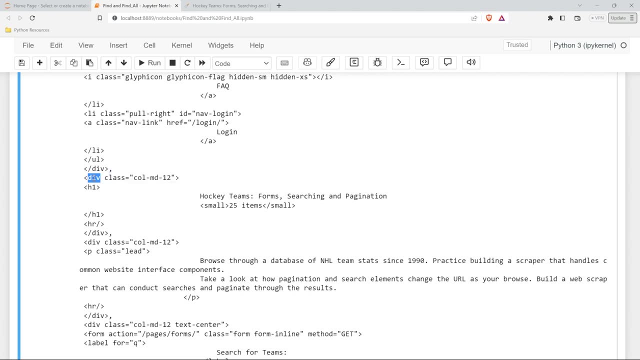 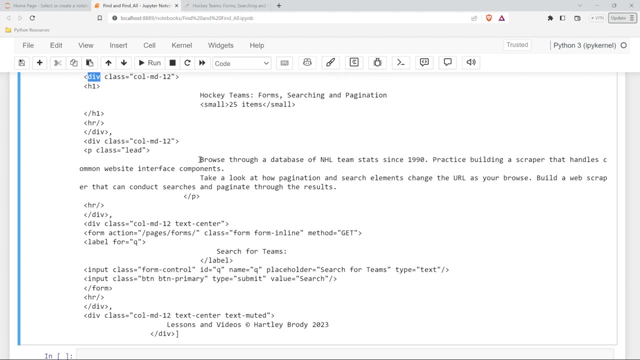 see it multiple times, something like right here, Or actually, let me see right here. So here's this comma, then here's our next one. So we have two of these div tags with a class of call dash MD, dash 12.. And in each of these we have different information. This: 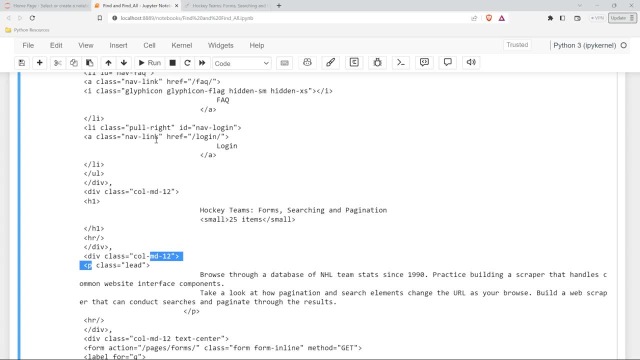 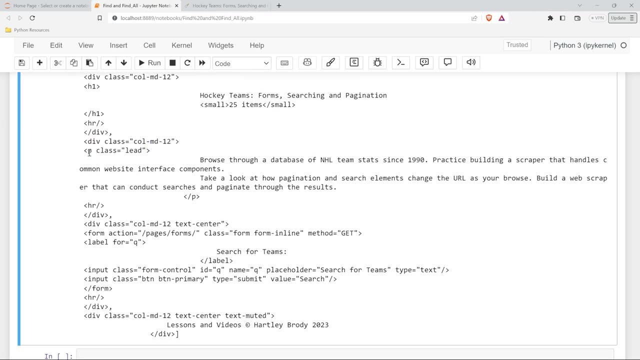 looks like a paragraph with this p tag right here And let's scroll back up. So I also think we should try out doing something like this p tag. Typically these p tags stand for paragraphs or they have text information in them. Let's try to p tag really quickly. 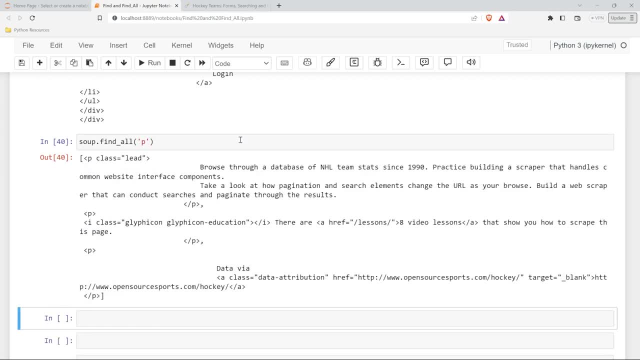 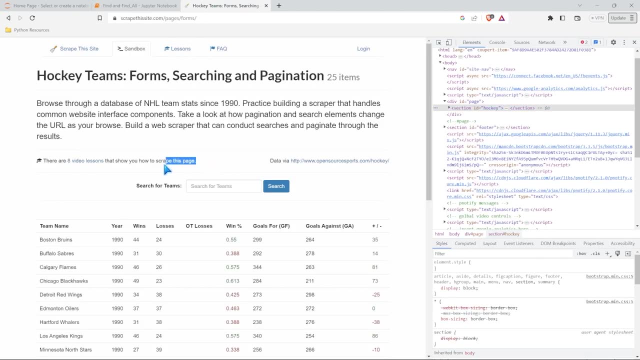 Let's just see what we get And let's run this And it looks like we get multiple p tags. Now, if we come back here, you can see that there's this information And it's this information that we're pulling in, And I'm just, you know, noticing that from right here. 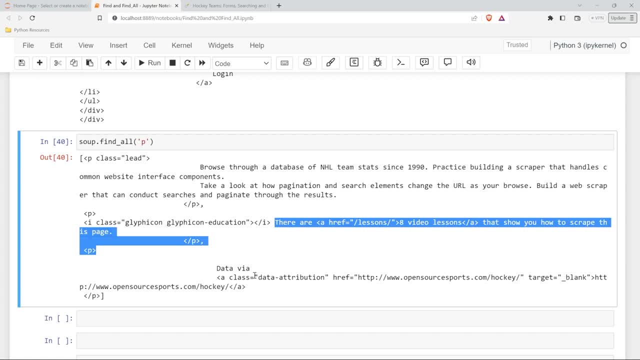 And then we have this information right here And it looks like there's one more, which is this h ref, which looks like this open source, So data via, and then that hyperlink or that link right there. So we have three different p tags. Now just to verify, and 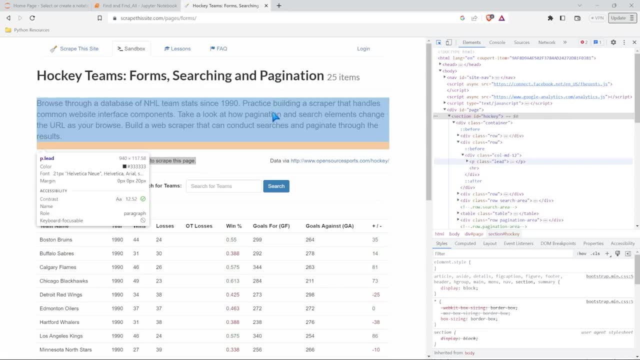 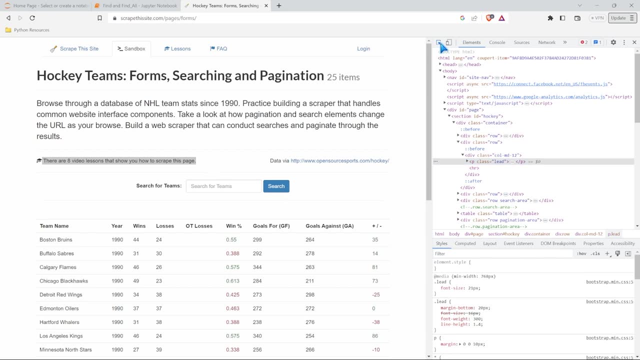 make sure that that's correct. we could do is come over here. we're going to click on this paragraph. it's going to take us to that p tag where the class is equal to lead. Come over here and look at this paragraph. Now we have another p tag right over here where 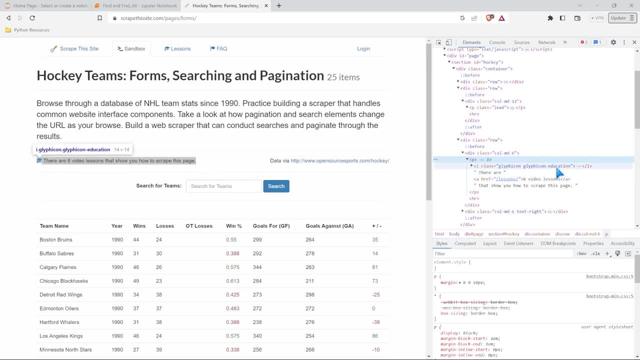 the class is equal to glyphocosm, glyphicon, glyphicon, slash education. I have no idea what that means. And then we'll go to our last one, which is right here, where the p tag is equal to, we have a tag h ref. 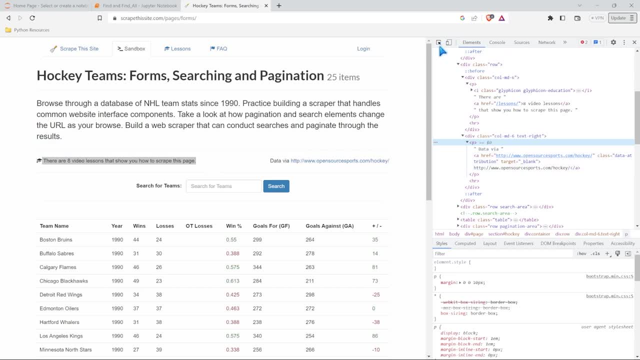 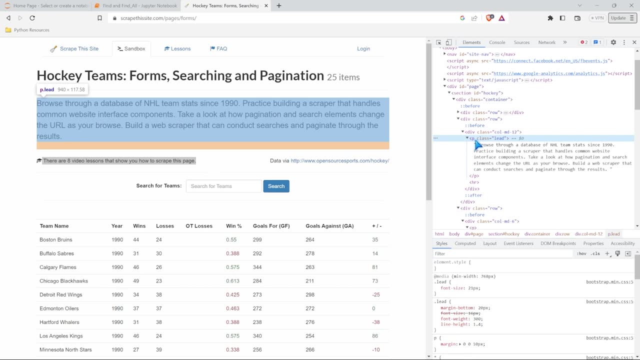 class and a bunch of other information. So let's say we just wanted to pull in this paragraph right here, let's go here and see how we can specify this information So it looks like p or the class is equal to lead, that looks like it's going to be unique to just that. 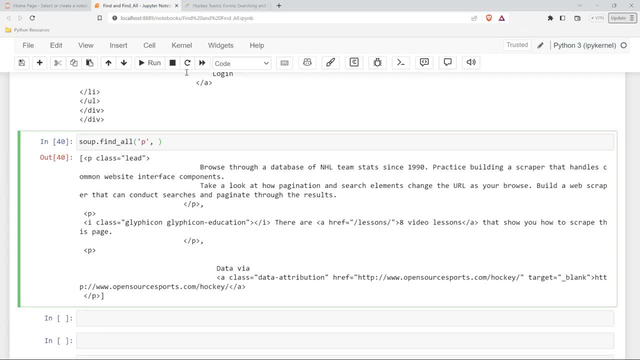 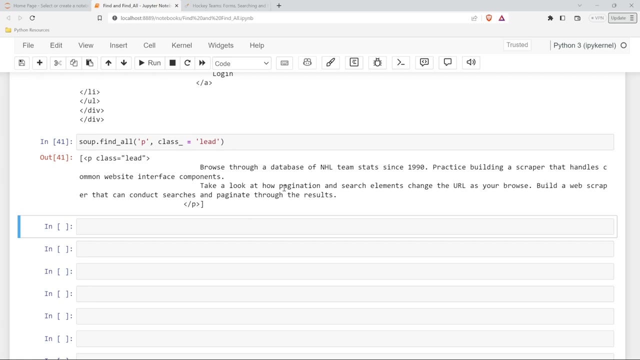 one. We're going to say comma and it was class, So you can do a class. underscore is equal to. and then we're going to say lead. Let's try running this And we're just pulling in that information. Now let's say we actually want to pull in this paragraph. 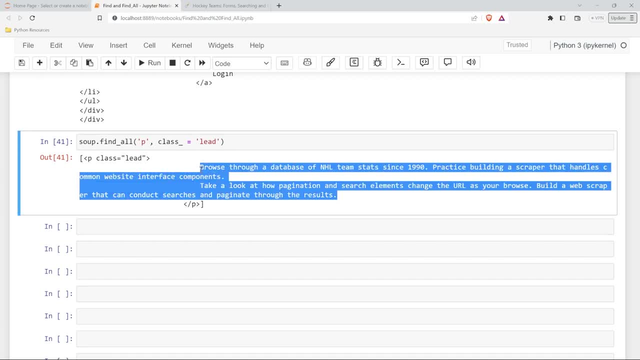 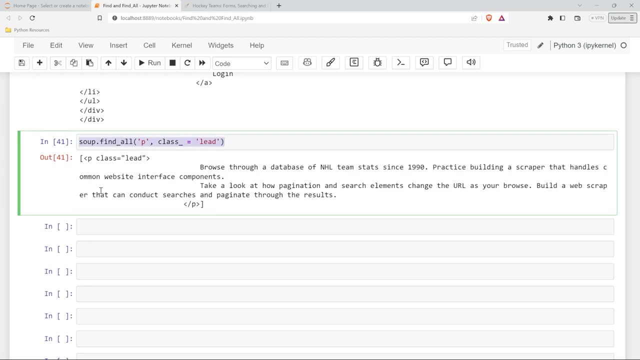 We actually want this text right here, And this is a very real use case. You know, let's say I'm trying to pull in some information or a paragraph of text. Well, let's copy this, And what we're going to then do is say dot text and let's run this: 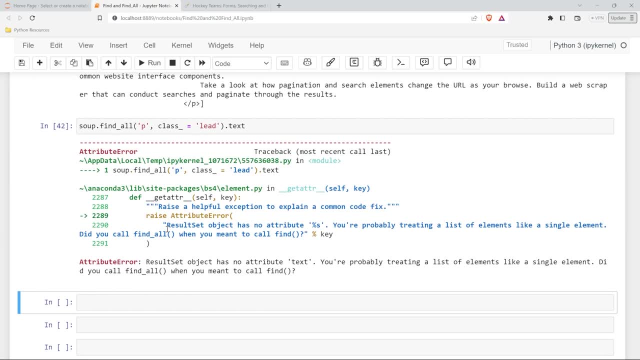 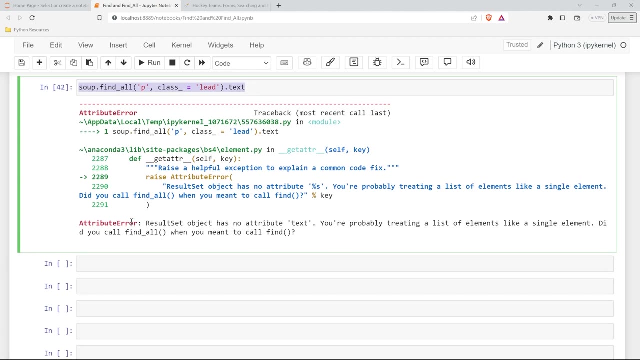 Now we're going to get an error right here- And this is a very common error- because we're trying to use find all. Unfortunately, find all does not have a text attribute. We actually need to change this to find. Typically, when I'm working with these find and find alls, I'm using find all most of. 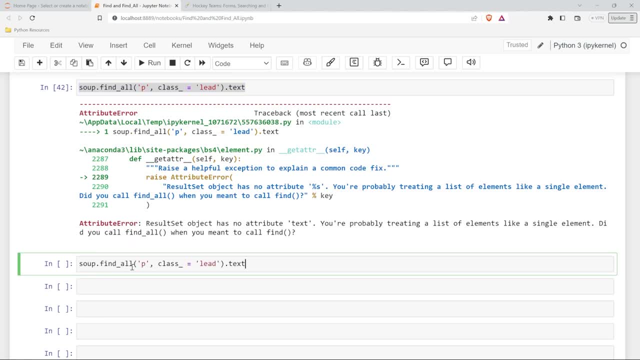 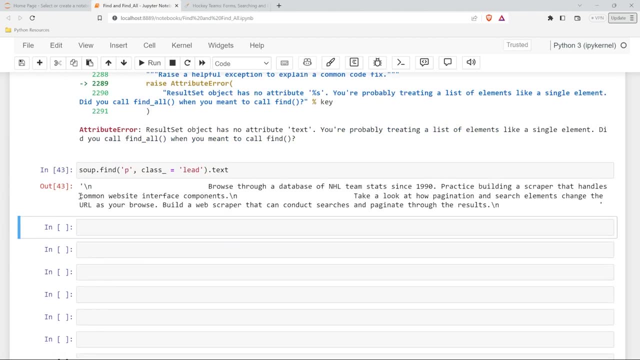 the time until I want to start extracting text. Then, when I specify it, I'll change this back to find Just like this: Now, let's try this. And now we're getting in parentheses this information. Now, this is all wonky and needs to definitely be cleaned up a little bit, but if we go back, 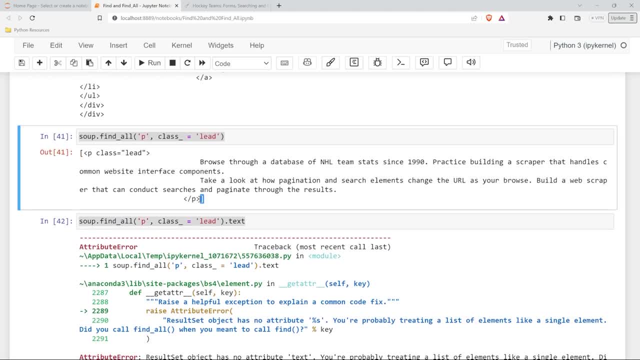 up. it's no longer in a list and we no longer have things like these P tags in here or this class attribute, So we're really just trying to pull out this information Now. again, this does not look perfect. We could even try to do something like dot strip. 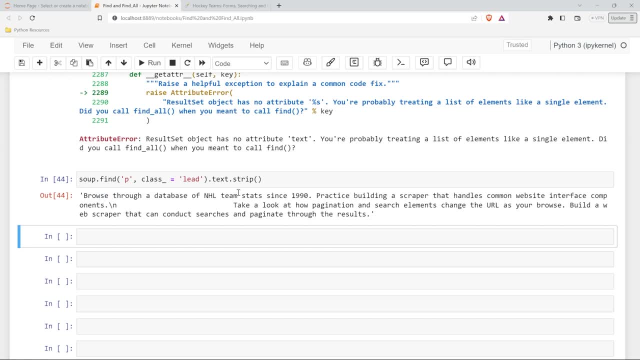 Look like there's some white space. Okay, Uh, that cleans it up a little bit. This definitely looks a little better, Um, and we could definitely go in here and clean this up more, but just for you know an example, this is how we can then. 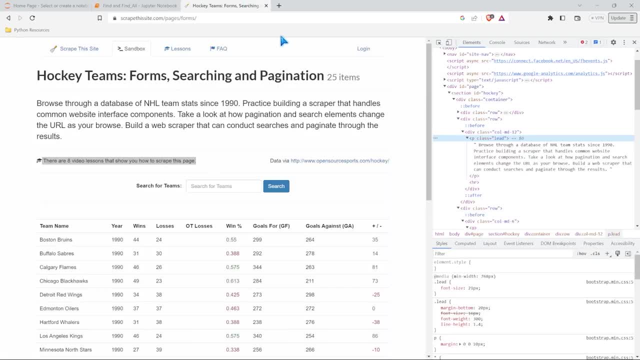 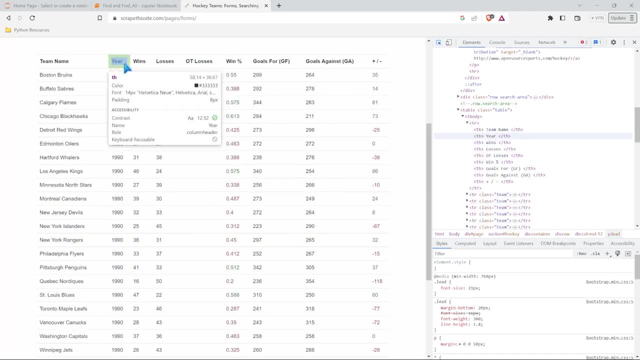 extract that information. Now let's look at one more example. This is some information and this is what we're going to do, Kind of our little mini project, in the next lesson on. let's say we wanted to take all this information. Well, what if we wanted to pull in something like the team name that's going to be in right here in this TR tag? 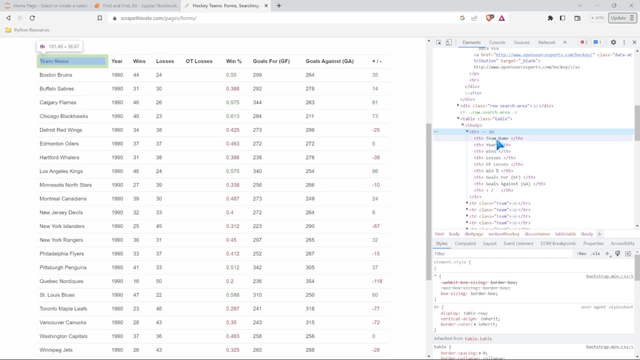 And each of these TR tags have TH tags underneath them. So if we scroll down, you'll notice that each row is this TR tag. So let's go ahead and search for, let's do TH, Let's just search for that first. 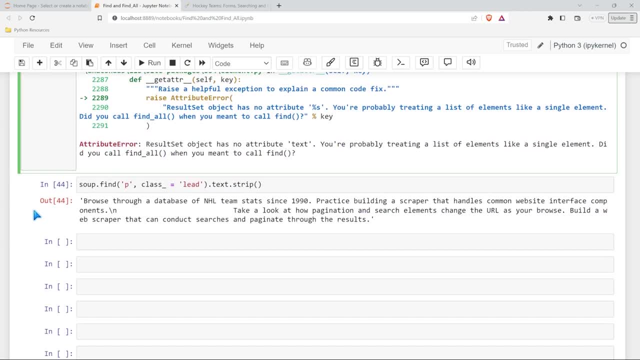 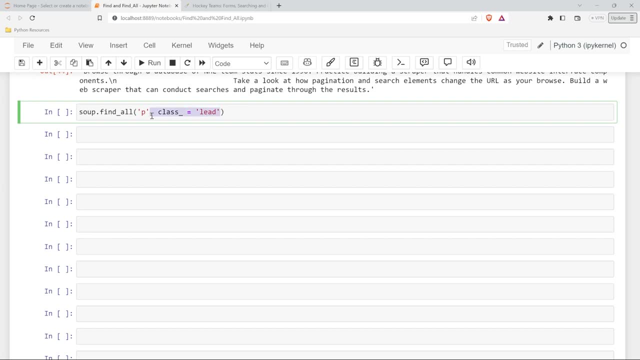 So let's come right back up here, Let's use this find all and we'll get rid of this text for right now, And let's just say we want to look for the TR that we said we were looking for. No TH. 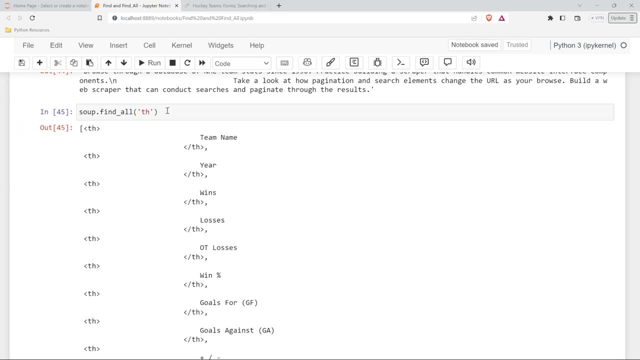 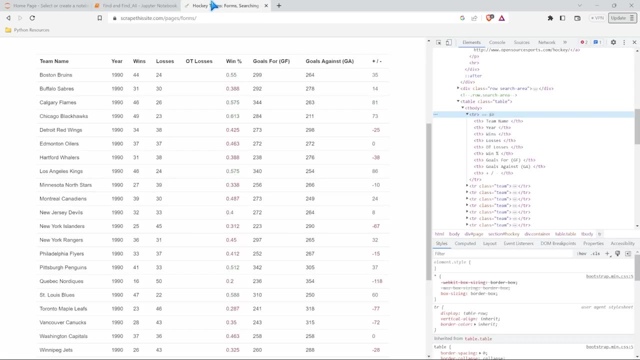 So let's say, we're looking for TH, Let's go ahead and run this, So we're going to have underneath this TH. we have team name, year wins, losses and notice: these are all the titles. So these titles are the only ones with these TH tags. 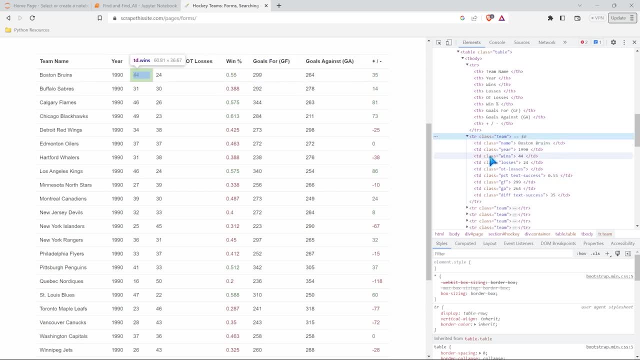 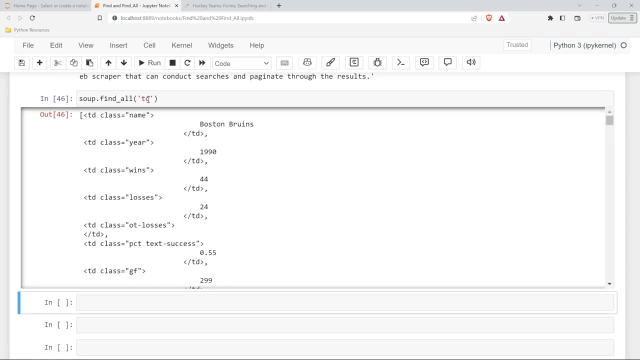 If we go down, you'll notice that the data is actually TD tags. So now let's go back and look for TD. We'll say D, and this is going to be a lot longer. We have a lot of information, but these are. 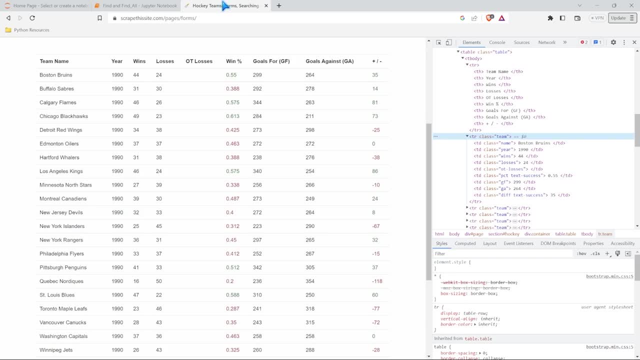 All the rows of data. Let's see if we can just get one piece of this data We're going to get back. We want just this team name. That's all we're trying to pull in for now, Um, and then we'll try to get this row. 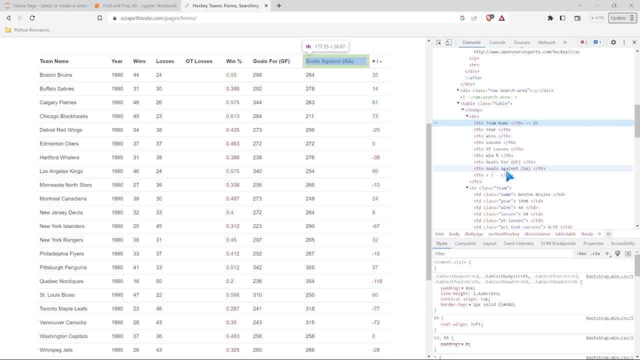 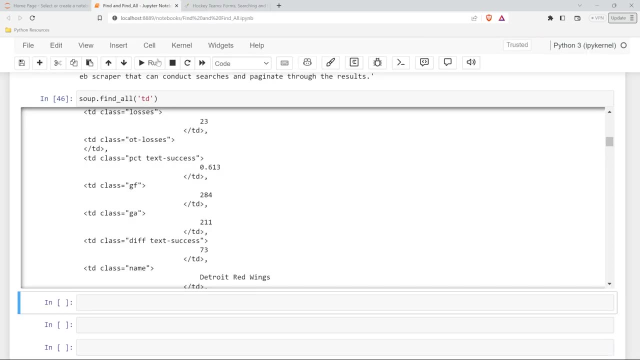 And then in the next lesson we're going to try to get all of this information, make it look really nice, And then we'll put it into a pandas data frame. So let's just get this team name right now. Let's go ahead. 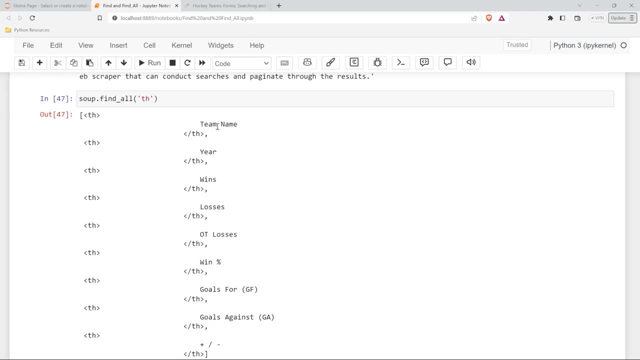 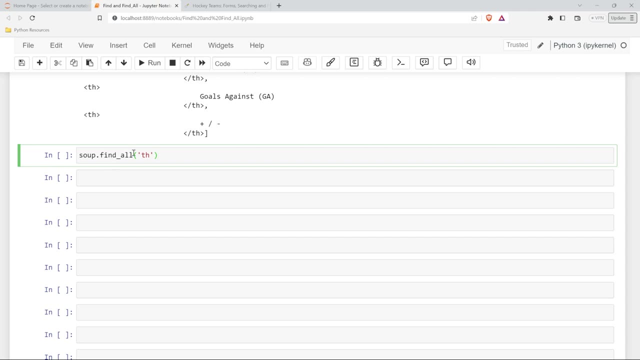 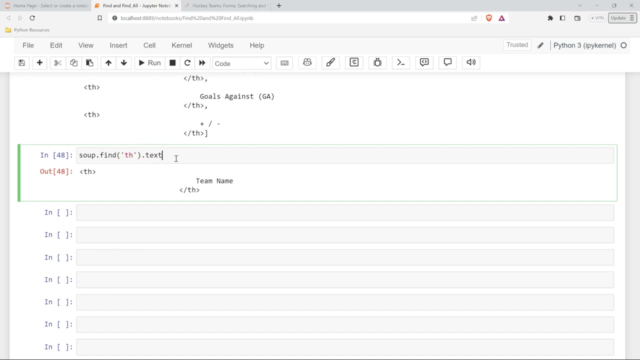 We're going to say TH, Let's run this. and we have this TH And now that we know we're Okay Getting this information in, we can do find: let's run this. So there's our team name. I'm just going to say dot text. 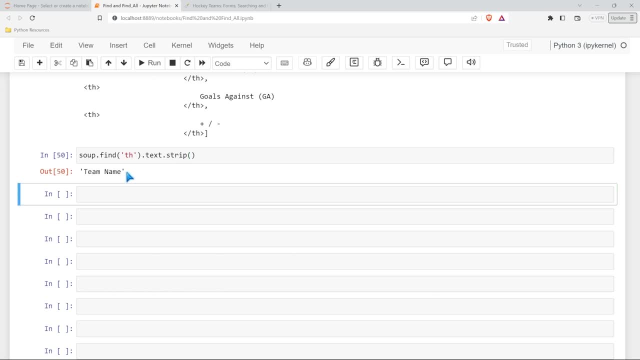 And again we can do dot strip just like that And bam, we have our team name. So you can kind of start getting the idea of how we're pulling this information out. We're really just specifying exactly what we're seeing in this HTML. 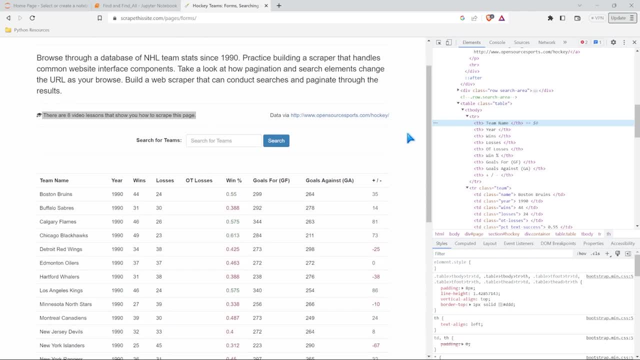 And what's really, really helpful in. you know, it's something that I do all the time Is I'm inspecting it and just kind of searching like how, what do I want, What piece of information do I want? 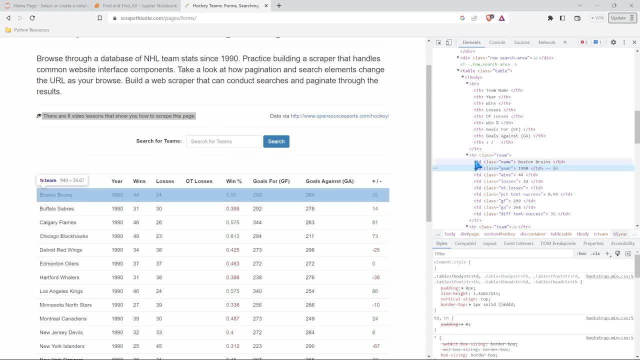 Then I go ahead and click on it and then I'm looking. you know where is this sitting in the hierarchy? It's within the body, It's within this table with the class of table. then it's down here where this TR tag and then this TD tag. 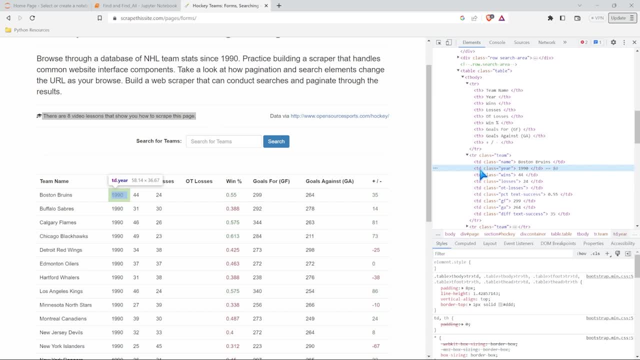 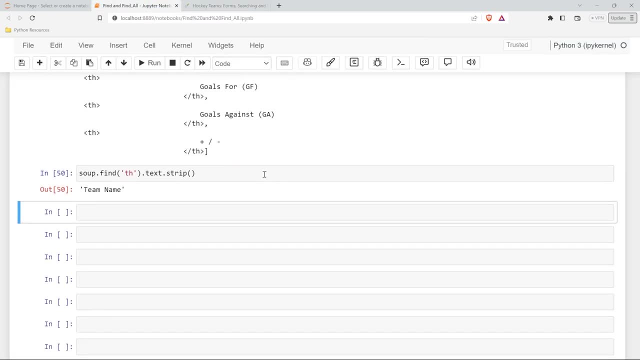 So I'm looking kind of at the hierarchy and I'm specifying exactly what I'm looking for. So that is what we're going to look at in today's lesson. That's how we can use find and find. all we were able to look at classes. 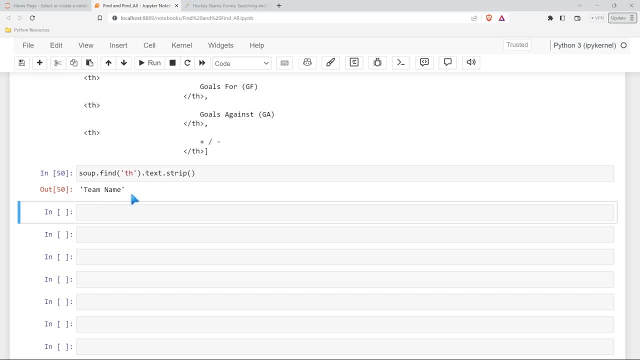 And tags and attributes and variable strings. which is this right here, getting that text and variable strings, and we will look at find and find all and how it's pulling that information in and how we can specify exactly what we're looking for now in the next lesson, which is definitely going to be the most exciting one, we're going to try to pull in all of this information.